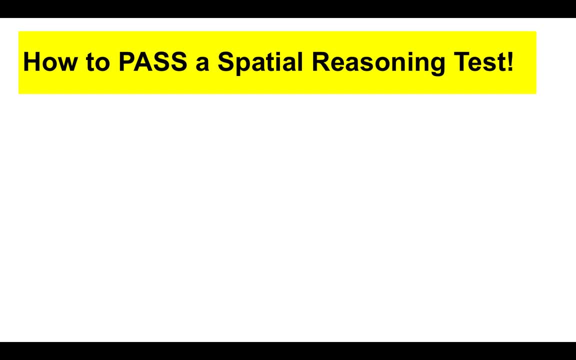 or constructed. So how do we pass a spatial reasoning test test? There is a three-step process to follow. Step number one: we need to learn the different types of spatial reasoning test questions that are commonly used during job assessments, And I will work through the different types during this tutorial. The second step is to 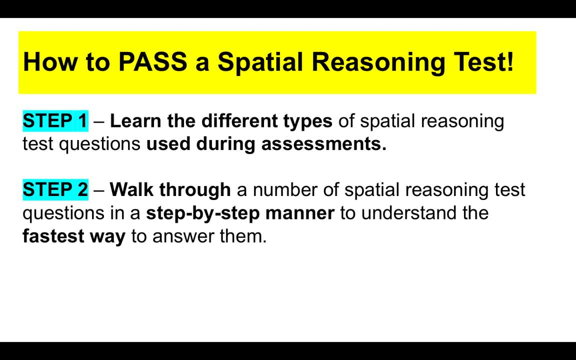 walk through a number of spatial reasoning test questions in a slow, step-by-step manner so that you can understand the fastest way to answer them Again. I will do that during this tutorial. And then step number three. You need to practice as many spatial reasoning test questions as possible, because the more 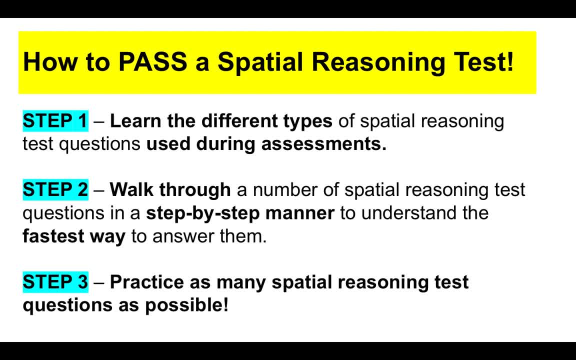 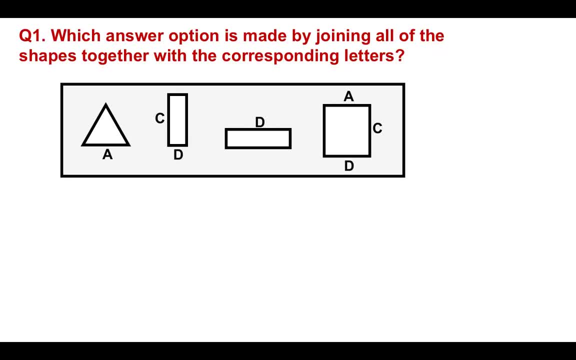 you practice, the better your scores will be, And I will tell you where you can get access to my online aptitude testing suite once we've completed the tutorial. So let's take a look at a number of sample spatial reasoning test questions. Question number: 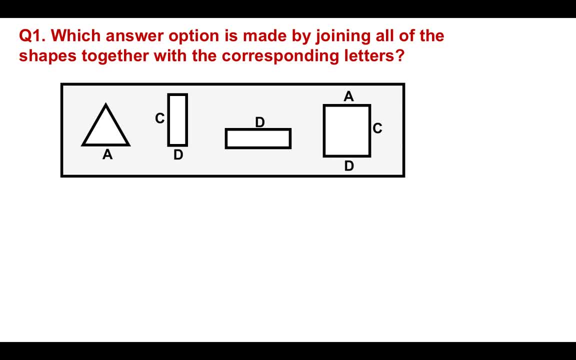 one which answer option is made by joining all of the shapes together with the corresponding letters is made by joining all of the shapes together with the corresponding letters. Is it A, Is it B, Is it C Or is it D? So what we have to do to answer this question is join the. 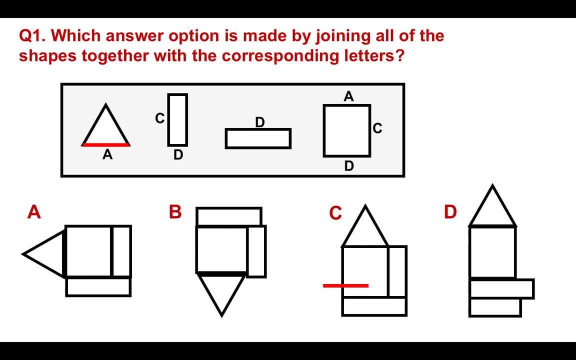 corresponding letters where they are shown exactly on each of the shapes. So we have the triangle there which would go on top of the rectangle, and then we would have the side of that rectangle that would fit at the side there and the top of that rectangle. 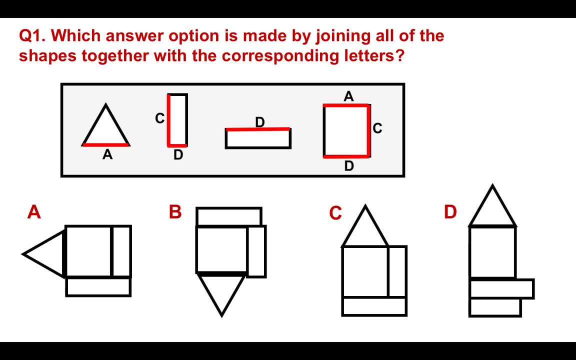 there would go on the bottom of that one, And that small one would also fit on the top of that rectangle too. So in your mind you have to visually construct these shapes with the corresponding letters. So if we take that triangle on the left, we then construct the. 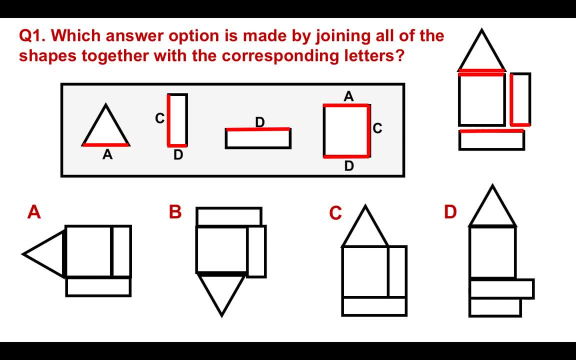 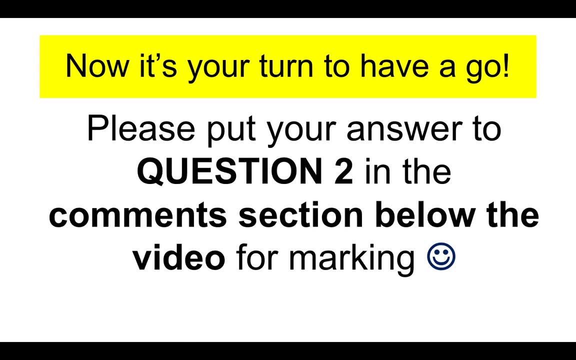 rectangle below it. We put C's together on the side and then D's at the bottom. So you'll be able to do this really quickly the more practice you undertake. So the correct answer there is, of course, C. So now it's your turn to have a go at one of these spatial reasoning test questions. 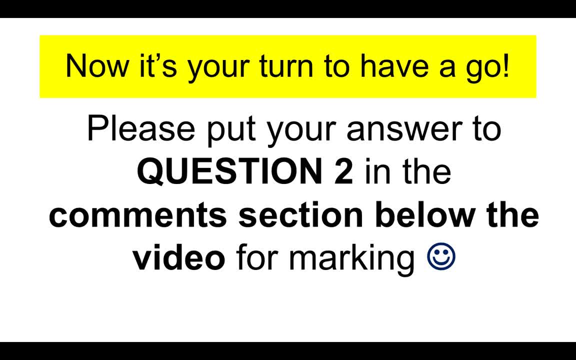 Please do put your answer to question number two in the comments section below this video for marking. We will come on it each day and mark them for you. Now on the question. I have put a timer on the right hand side. You've got about 13 seconds to answer each question. 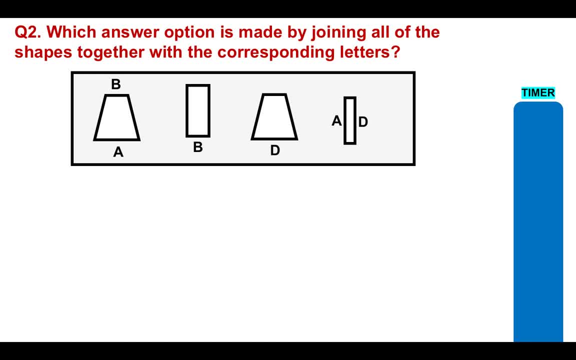 So I'm putting you under a little bit of pressure. Let's see if you can do it within the time allocated, And then that will enable you to improve your scores. So question two: which answer option is made by joining all of the shapes together with the corresponding letters? Is it A, B? 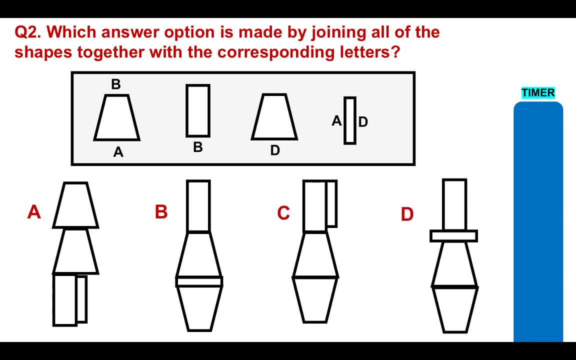 C, D. Put your answer in the comments section below the video. Here's the timer. OK, well done. Now if you need a little bit more time, please do feel free to pause the video. It's important you work out the correct answer. Have another go, So please. 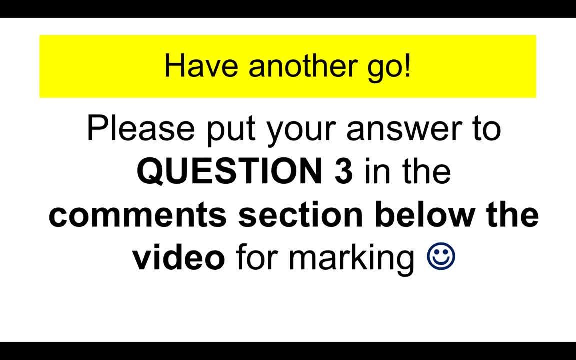 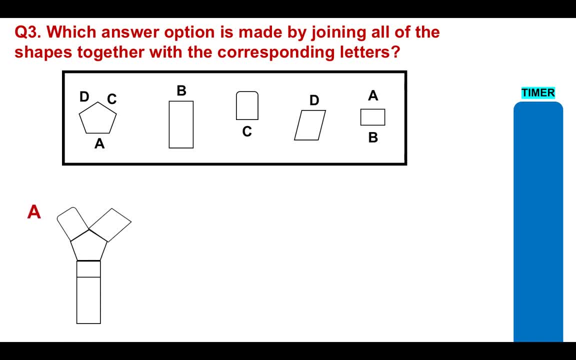 put your answer to question number three in the comments section below the video for marking Which answer option is made by joining all of the shapes together with the corresponding letters. Is it A, B, C or D? Here's the timer, OK. 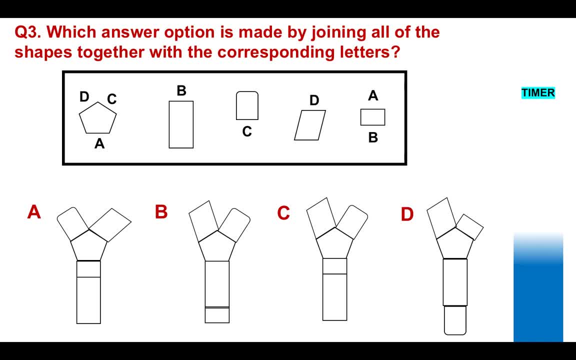 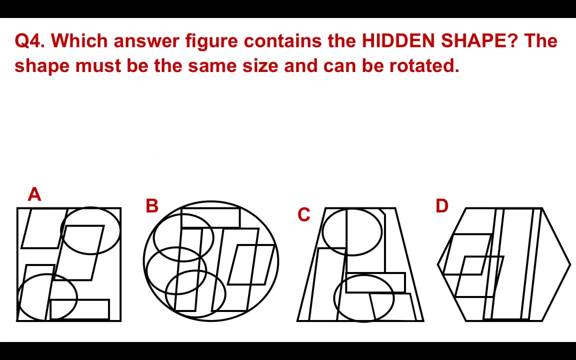 Well done. Let's move on to a different type of spatial reasoning test question, this time Question four. Which answer figure contains the hidden shape? The shape must be the same size, but it can be rotated, So there is the hidden shape. Which answer figure A, B, C? 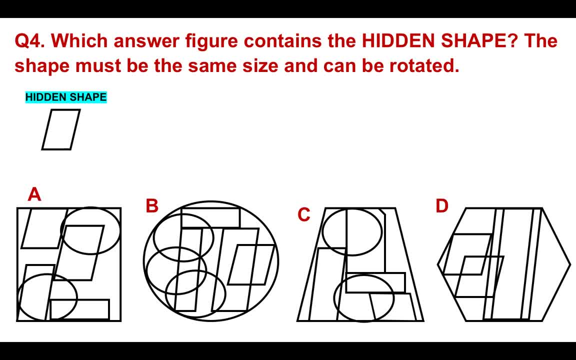 or D contains that hidden shape. OK, The hidden shape must be the same size, but it can be rotated. So don't forget, we can rotate that shape. So we're looking for either of those two shapes from the answer options of A, B, C or D, And I can straight away notice that it is there at the bottom of C, So the 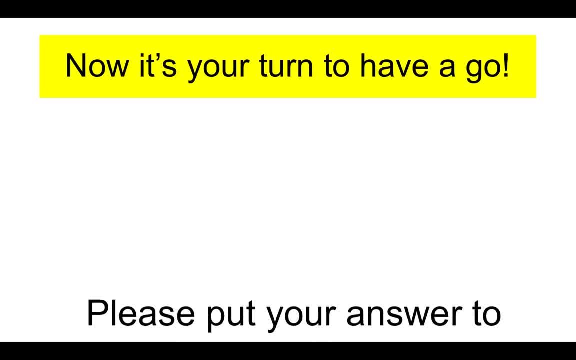 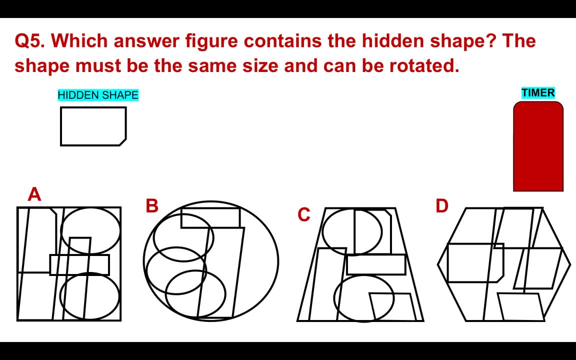 correct answer, there would be C. So now it's your turn to have a go. Please put your answer to question five in the comments section below the video for marking Question five. Which answer figure contains the hidden shape? The hidden shape contains the hidden shape Which. 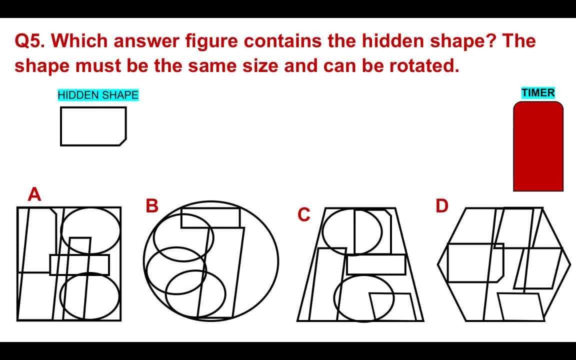 answer. figure contains the hidden shape. The shape must be the same size, but it can be rotated. Here's the timer. OK, Brilliant, Well done. Don't forget: if you are enjoying this video, which I hope you are, please do give the video a LIKE. That then tells me that you enjoy the content. 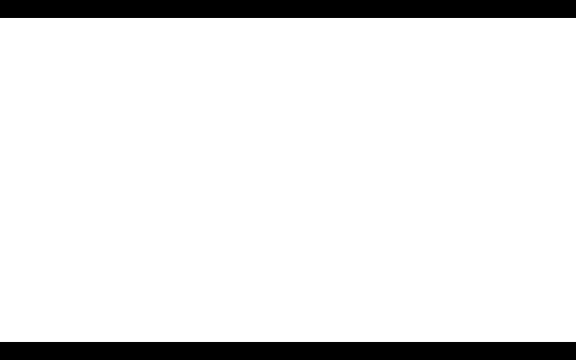 Thank you. Let's now try a different type of spatial reasoning. test question Question number six: Which answer option is a top-down 2D view of that question figure? So there's the question figure. Which answer option is a top-down 2D view of the question figure? 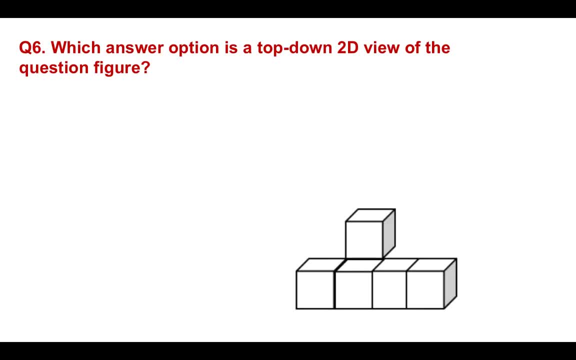 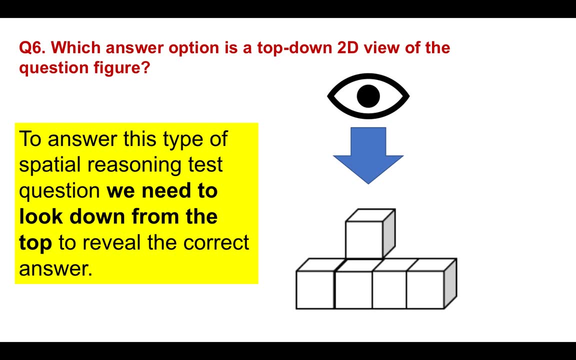 Is it A, B, C or D? So, in order to answer this question, what we have to do is we need to look down from the top to reveal the correct answer. So you have to imagine that you are looking down on the top of that question. Do you want to see the left, the right or the? 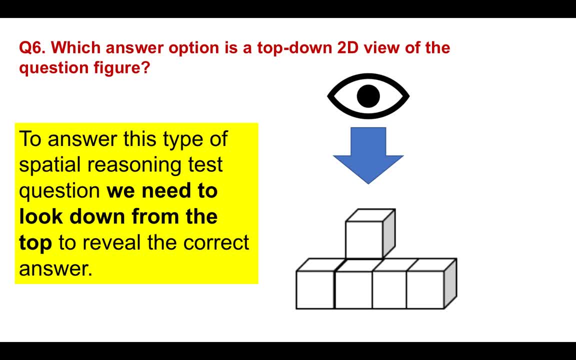 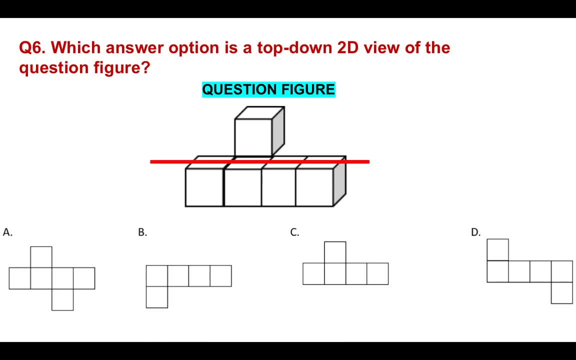 top of that 3D set of cubes And that will give us the 2D option. So the 2D option is A, B, C or D, And we can see there that there is a row of four cubes And the second one. 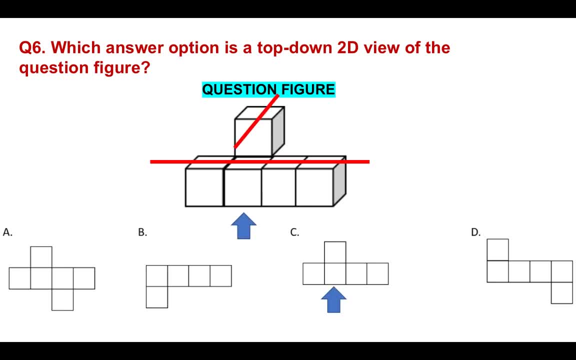 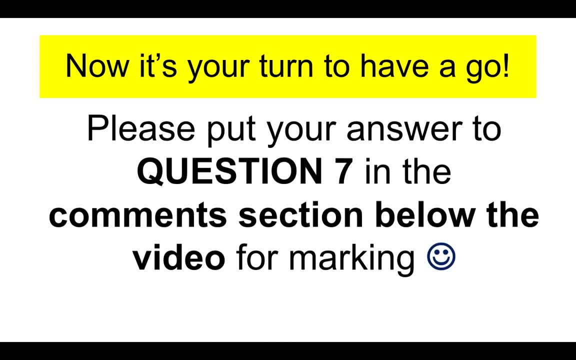 along. there is one to the right, And the only one that has one to the right there, and nothing else, is C, So the correct answer is C. So now it's your turn to have a go at one of these questions. Please put your answer to spatial reasoning test, question number. 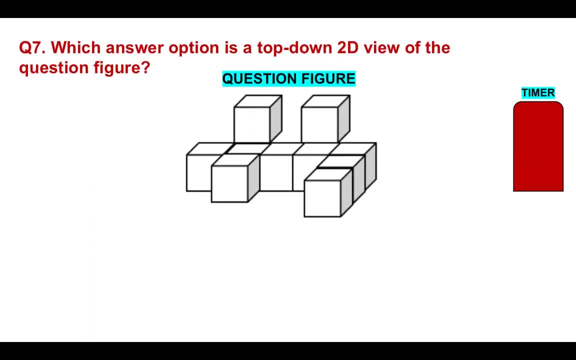 seven in the comments section, below the video for marking Which answer option is a top-down 2D view of the question figure. Is it A, B, C or D? And here's your timer. OK, Fantastic, Well done. Let's now try a different type of spatial reasoning. 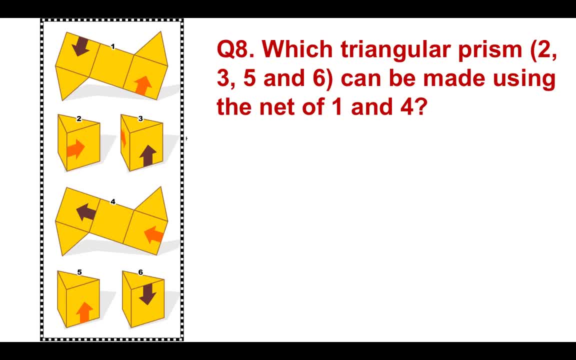 test. test question. Let's make them a little bit harder. Question number eight: Which triangular prism can be made using the net of 1 and 4?? I'll just quickly repeat that: Which triangular prism can be made using the net of 1 and 4?? So these are the triangular 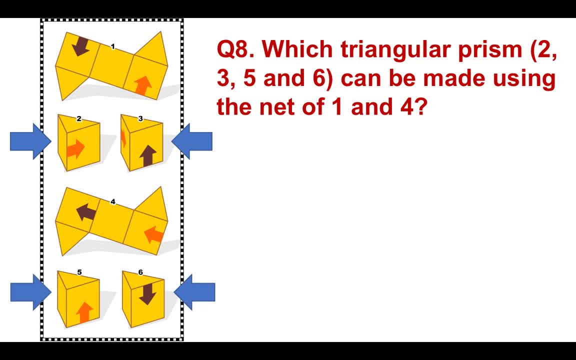 prisms, Which one of them can be made from either of the nets or net 2?. So the best way to tackle this type of question is to do a process of elimination to work out which ones they are not. So if we look at the first net, we can see that 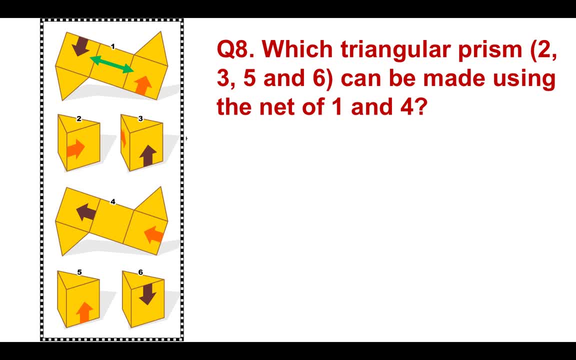 there is a gap between those two shapes, the orange arrow and the brown arrow, and the same on number four. Therefore it cannot be three, because you've got two arrows close together. There needs to be a gap between them, so it's not three. Then, if we look, 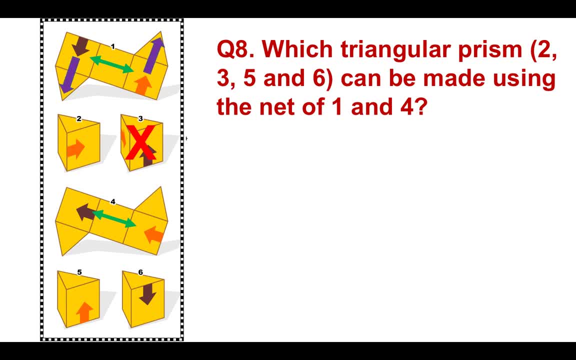 at that orange arrow: it's pointing to the top of the triangle, and the same with the brown one there, And then the orange one is pointing to the left, and that one is also pointing to the left- sorry, to the right- if you put it up the correct way. So therefore we can see that it's not number. 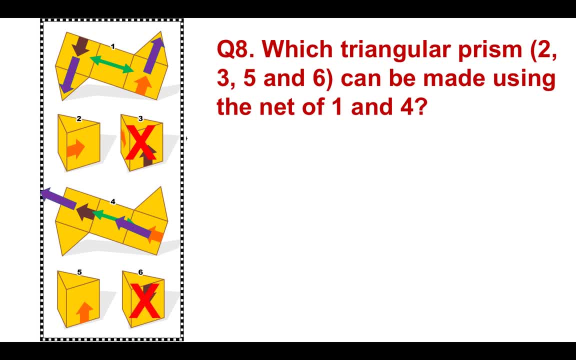 six, because that brown arrow is pointing down and it should be pointing up, And you can also look at that orange one pointing to the right there, when the orange one is actually pointing to the left. So it's not number two. Therefore, through a process of 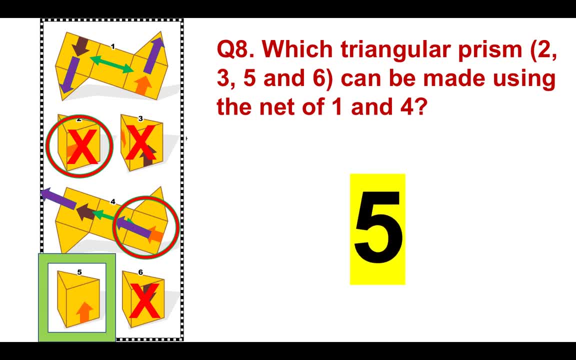 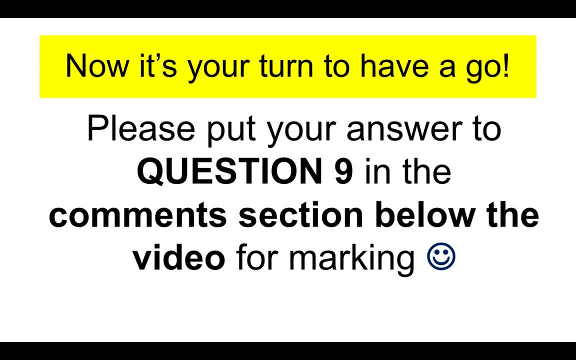 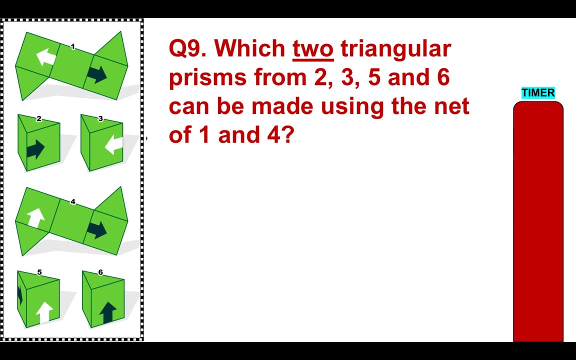 elimination. the correct answer is three. That is number five. So now it's your turn to have a go. This is a tough one. Please put your answer to question nine in the comments section below the video for marking Question nine: Which two triangular prisms from two, three, five and six can be made using the 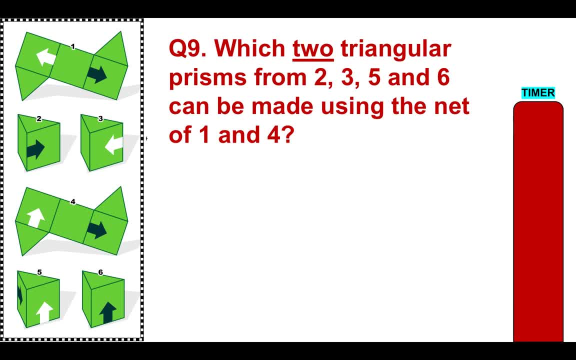 net of one and four. So you're looking for two answer options, Which two triangular prisms from two, three, five and six can be made using the net of one and four. Please put your answer in the comments section below. Here is the timer. 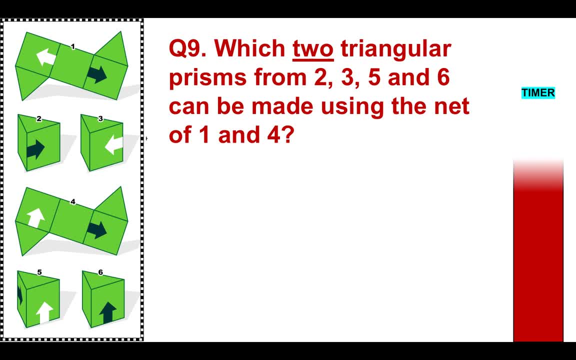 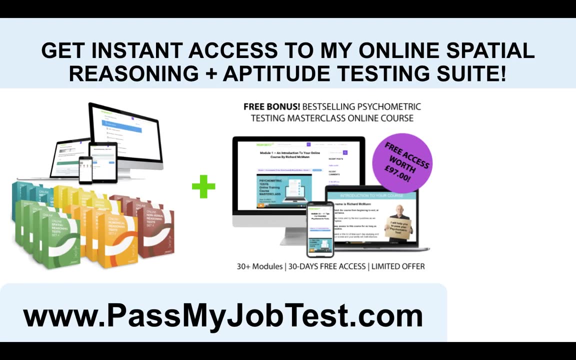 Okay, Brilliant, Well done. So don't forget. step number three was to practice lots of spatial reasoning test questions, and I have the perfect resource for you. If you click the link in the top right-hand corner of the video, it will take you through to my website. 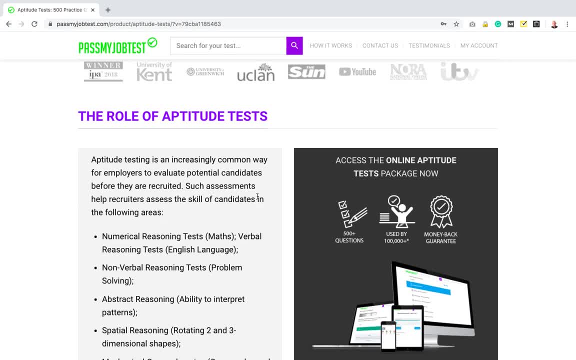 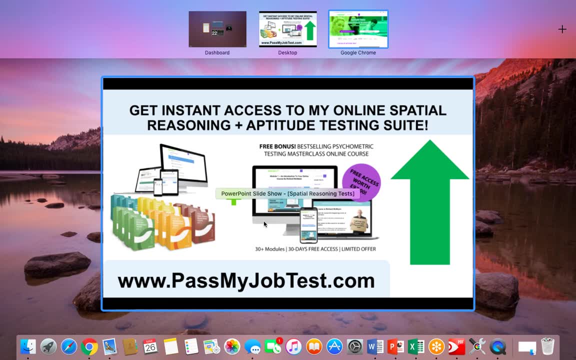 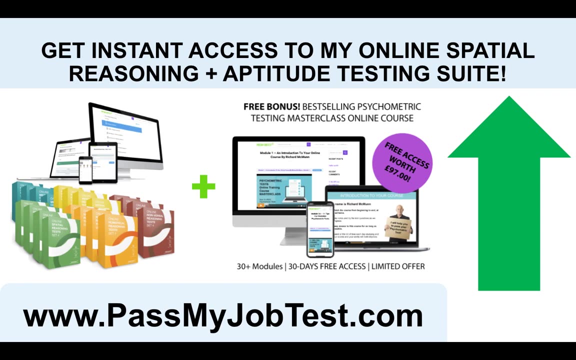 here, PassMyJobTestcom, You can get instant access to 500 plus aptitude test questions, including lots of spatial reasoning test questions. So click that page, Have a look at my online access. You can get access to the testing suite on your phone, your laptop, your computer and you get unlimited. 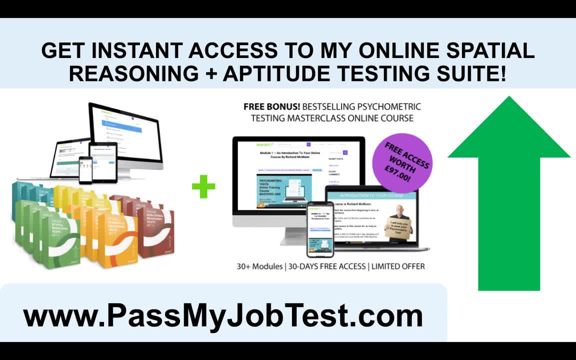 access to it, So please do give that a try. Thank you very much for watching. Don't forget to subscribe to the channel and please do hit the like button. I would very much appreciate your support, if you did, And don't forget to put your answers in the comments section. 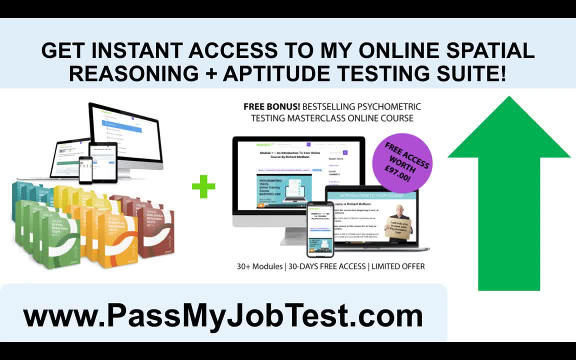 below And we will come on it each day and answer them for you. Thank you very much, And I wish you all the best for passing your spatial reasoning test. 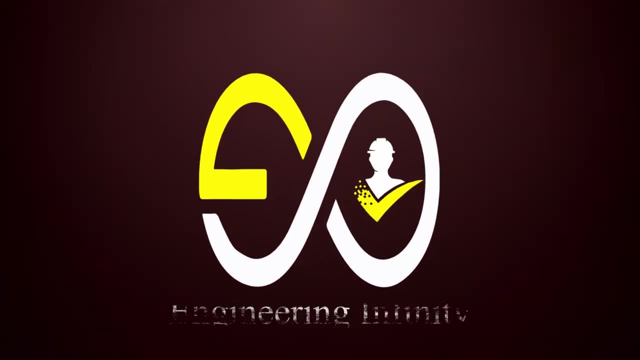 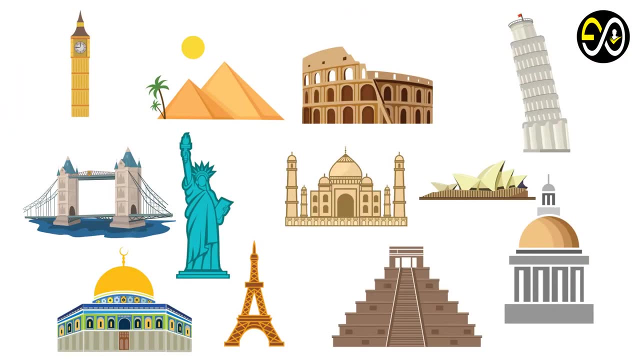 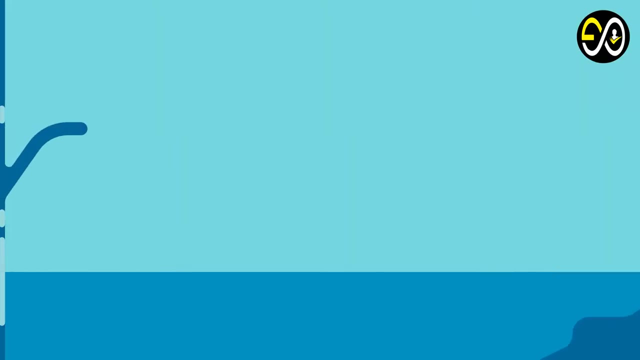 Everyone is aware of the Empire State Building, Burj Khalifa or the Eiffel Tower. Historical monuments like the Great Pyramids and the Leading Tower of Pisa are usually identified by their enormous height, But do you know how to measure the height of such a building? 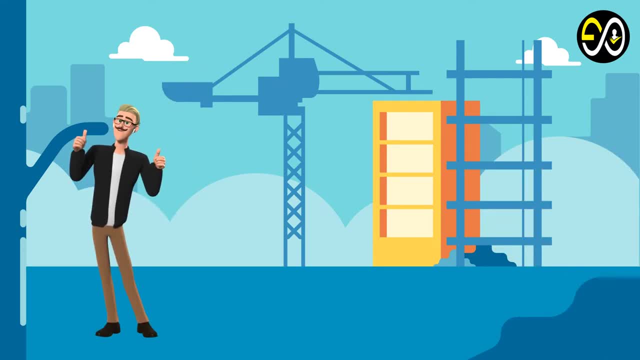 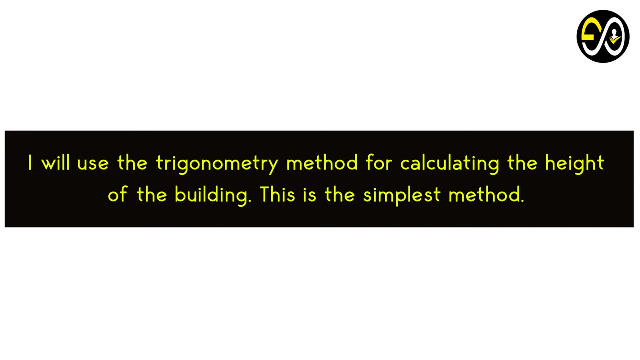 Sometimes we may need to find out the height of a building before or after construction. In this video, I will use the trigonometry method for calculating the height of the building. This is the simplest method. You can use this method to find out the height of any objects. 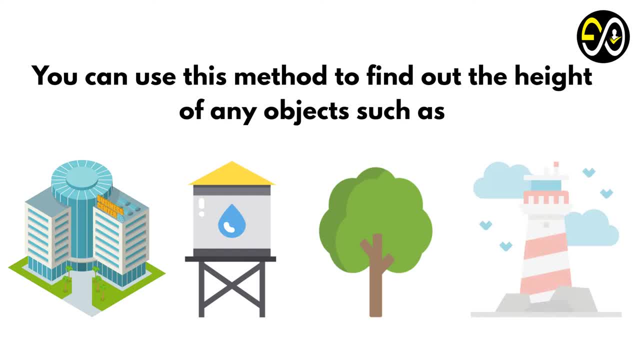 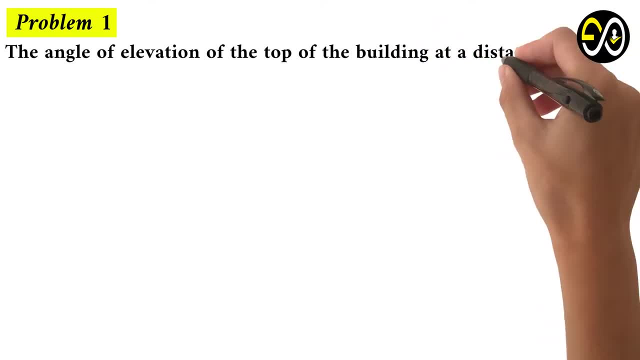 such as towers, water tanks, trees, lighthouses, etc. The angle of elevation of the top of the building at a distance of 50 meters from its foot on a horizontal plane is found to be 60 deg. Find the height of the building. 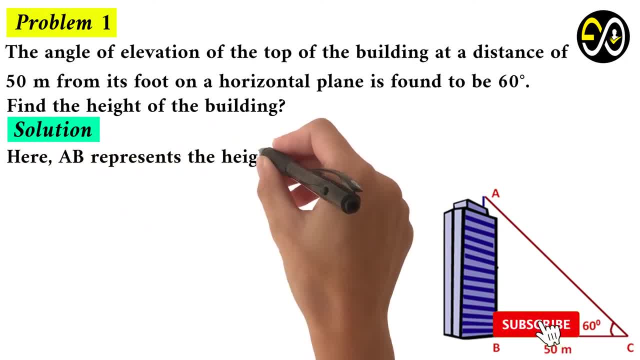 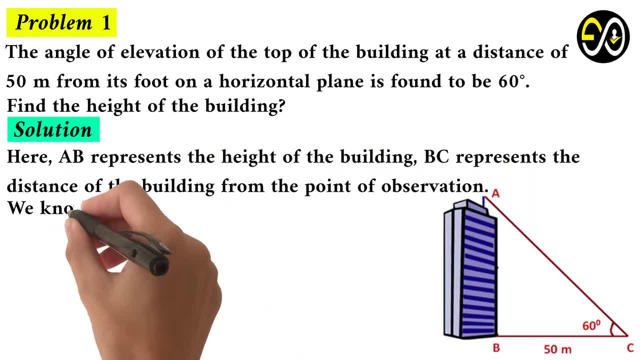 Here a b represents the height of the building, b c represents the distance of the building from the point of observation. We know tan theta equals opposite side over adjacent side. tan 60 deg equals ab over bc. Square root of 3 equals ab over 50.. ab equals 86.6.. 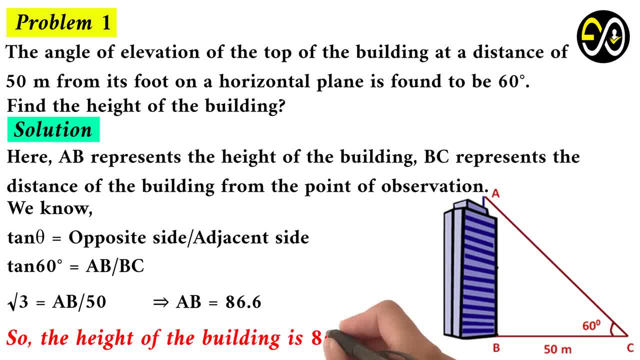 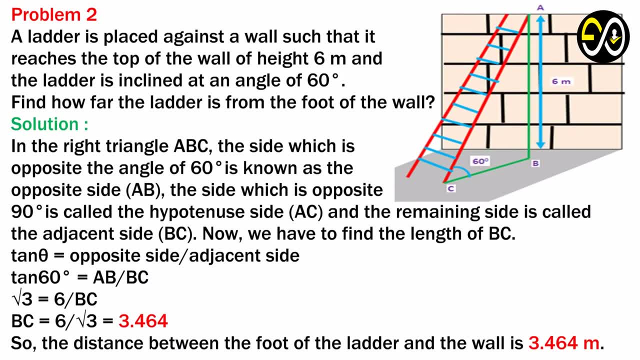 So the height of the building is 86.6 meters. The angle of elevation of the top of the building is the same as the height of the building. So the angle of elevation of the top of the building is the same as the height of the building. 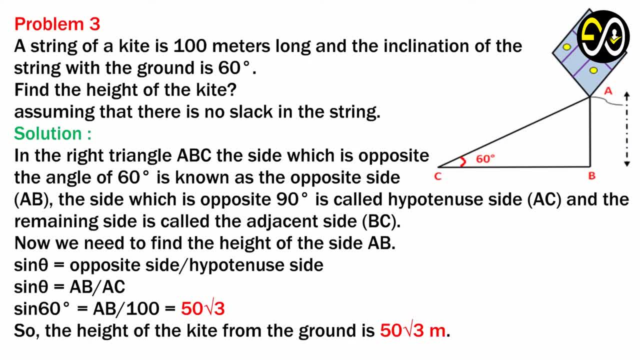 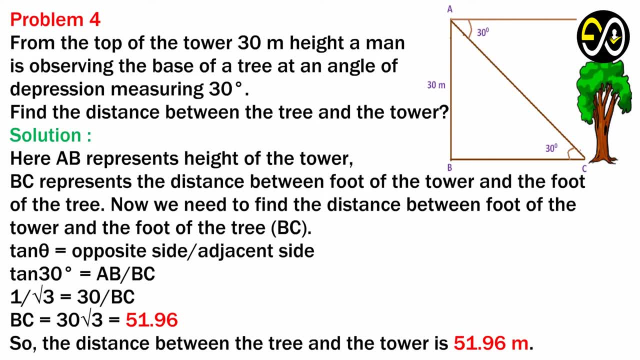 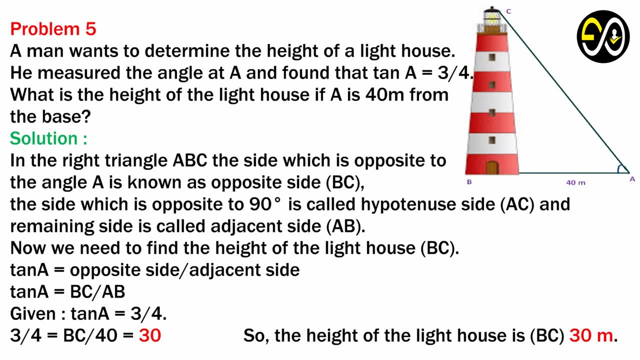 Let's go to the top of the building. In this part I will use the trigonometric method. In the first part, the height of the building is considered to be the愚ür. The further the height is, the greater the building will be.